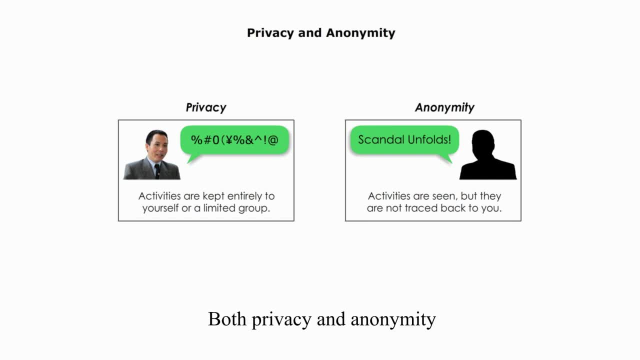 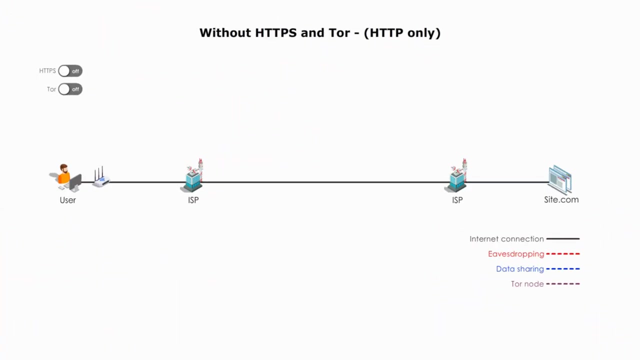 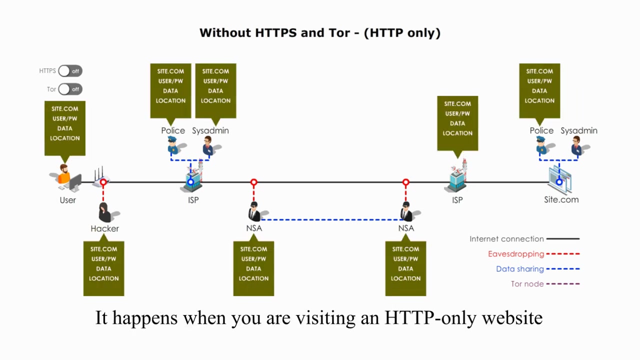 the right to privacy. Both privacy and anonymity are necessary and crucial to a free society. Today, my topic is the protection of online privacy and anonymity with HTTPS and Tor. The first scenario is HTTP-only traffic. It happens when you are visiting a HTTP-only website with one of the major web browsers. 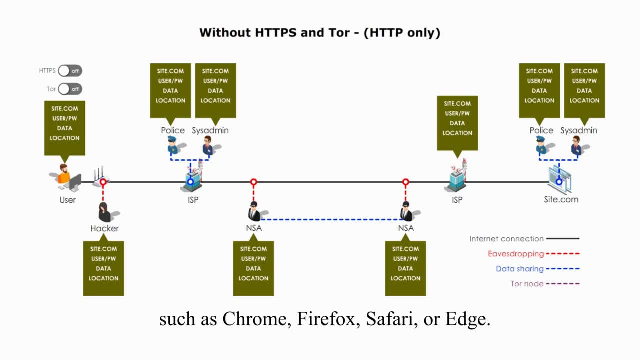 such as Chrome, Firefox, Safari or Edge. HTTP means your data is transported in a specific way. In this situation, you would be visible at any point to anyone. Hackers cops. your internet service provider, ISP national security agency. 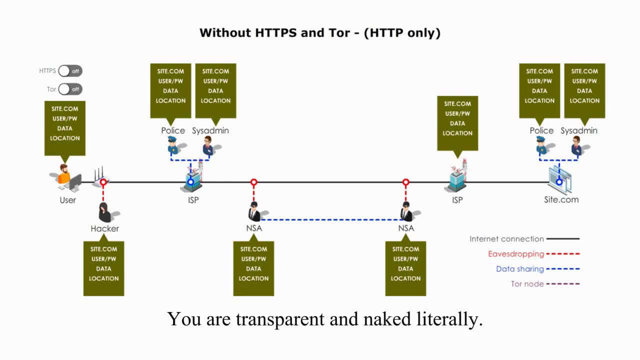 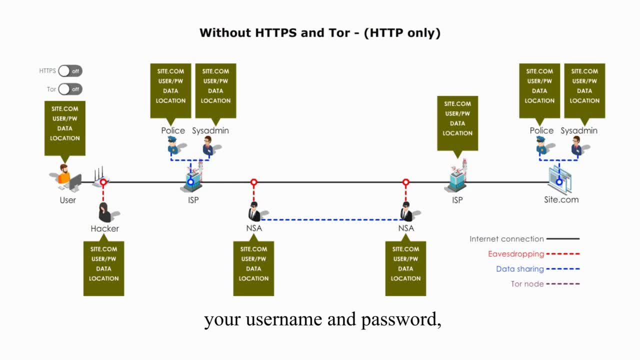 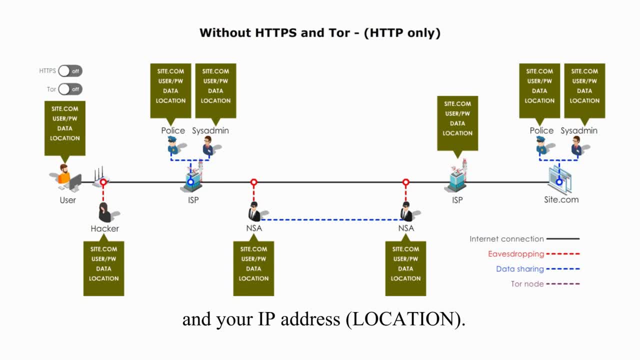 and your IP address location. The second scenario is HTTPS-only. HTTPS means your transmitting data is encrypted. HTTPS-only can protect your data- your username, password- in the middle, thus protecting your privacy, even though they may still know your IP address, your location and the site you are visiting. 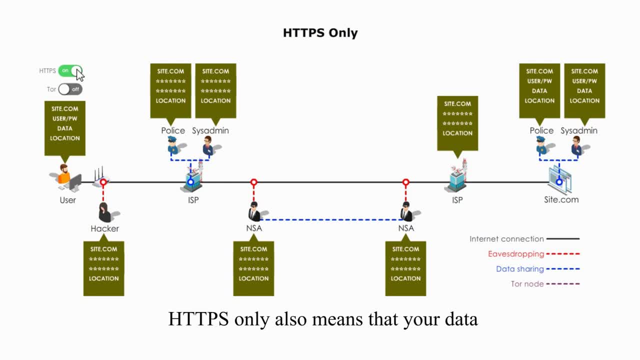 HTTPS-only also means your data may be vulnerable at two endpoints: the client-side, you and the web server. The third scenario is using Tor only. It means that you are using the Tor browser to visit an HTTP-only website. The Tor network hides your traffic, but once you leave the Tor network, your traffic and